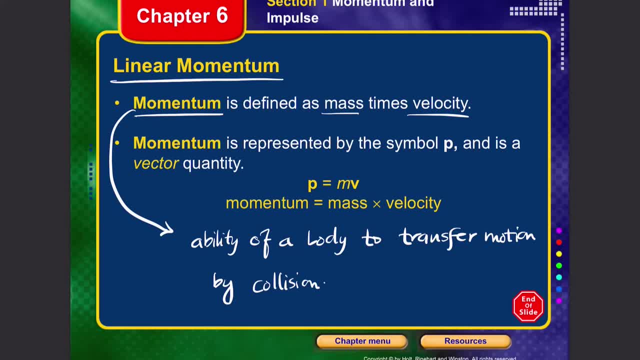 So momentum in simple sense is the ability of a body to transfer motion by collision. So momentum in simple sense is defined as mass times velocity, and it's still a vector quantity because velocity is a vector quantity. So you are multiplying a scalar with a vector, so we can consider that the original quantity will also be a vector. 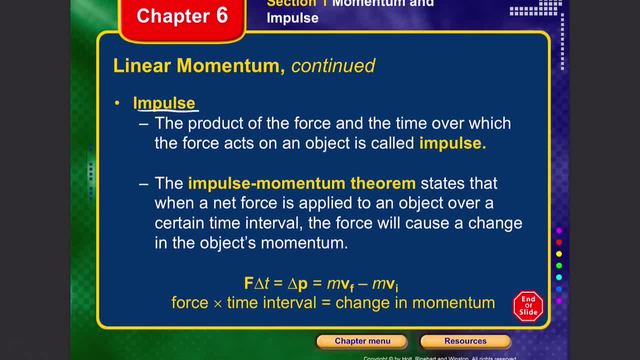 Next. so next let's talk about another form of momentum, called impulse. So impulse is the product of force and time over. so the product of force and the time over which the force acts on an object is simply called impulse. So we use what we call the impulse momentum. 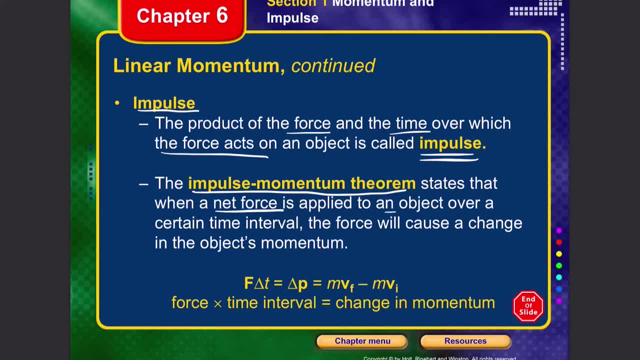 theorem to state whether a net force. when a net force is applied to an object over a certain time interval, the force will cause the force to move in a certain direction. The force will cause a change in the object's momentum, So it can be written as force times. 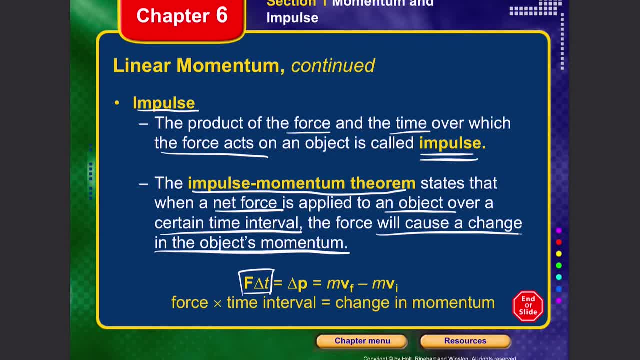 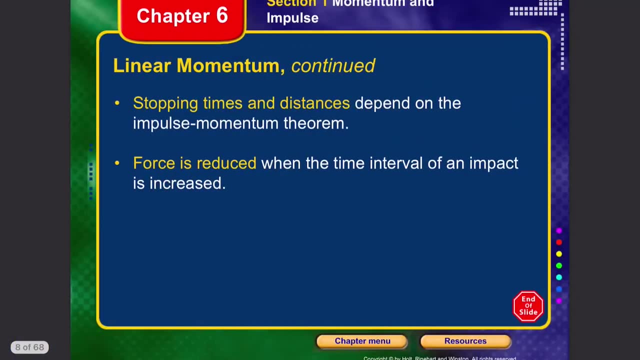 delta t or force times f times delta t equals the change in momentum. So change in momentum is called impulse and it's written as pf minus pi, final momentum minus initial momentum, So which is basically mvf minus mvi. Now stopping times and distances generally. 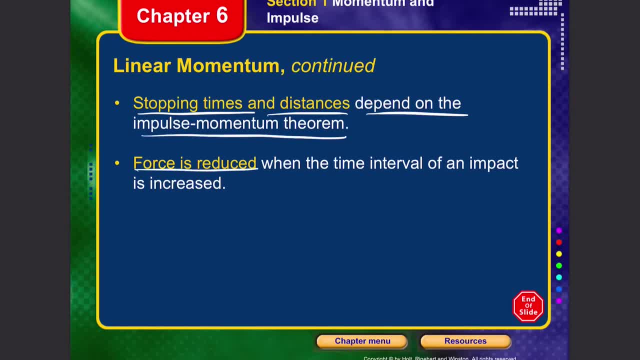 depend on the impulse momentum theorem and generally force is reduced when the time interval of an impact is increased. So think about the change in momentum delta p as force into time. So if the time is less, then there is a high amount of force. If the time is more, 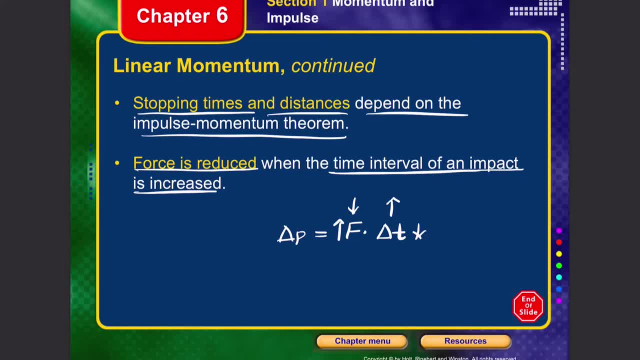 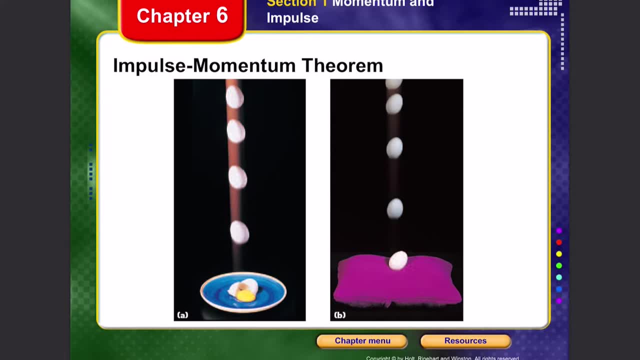 if there is more time, which means that the amount of impact force is less. So this is much more understandable. if you look at, let's say, you know if you're dropping an egg onto a plate and if you're dropping an egg onto a pillow. 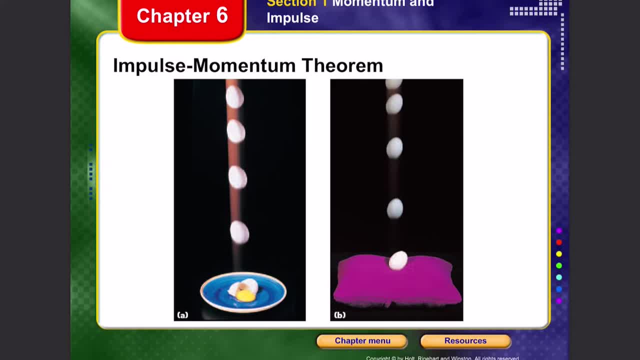 Now notice that when you're dropping the egg onto a plate, the impact time that it takes, the amount of time it impacts the plate- is really less. So in this situation, time here is much less So, which means the amount of force here is very high, So resulting in the 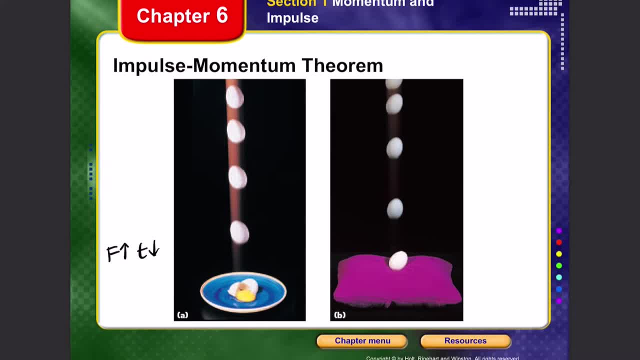 egg breaking, But when you're putting a pillow, the amount of impact time increases rapidly, while the force decreases. Notice that the p here stays constant. The change in momentum is still constant. The only thing that changes is the impact time resulting in the change. 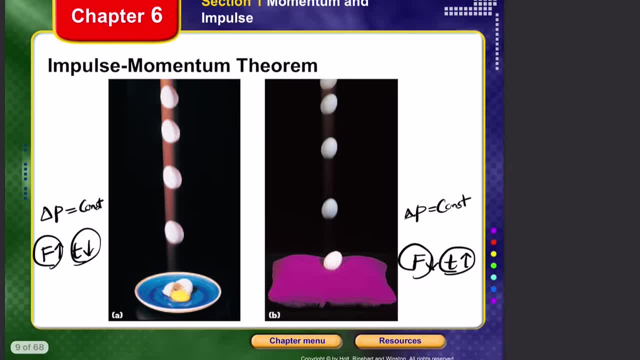 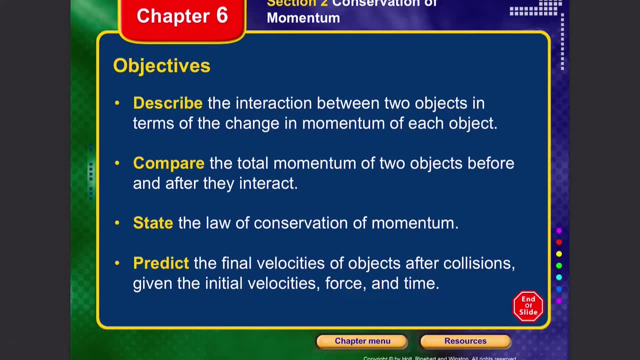 in the impact force. So this is the idea behind the impulse momentum theorem. So with that, that is momentum. Next, let's talk about conservation of momentum. So in conservation of momentum, we're going to try to describe the interaction between two objects in terms of change in momentum. 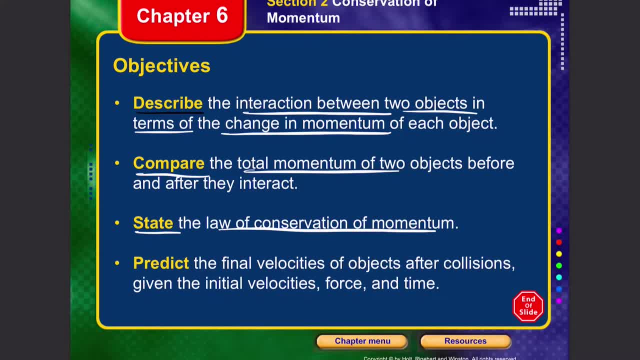 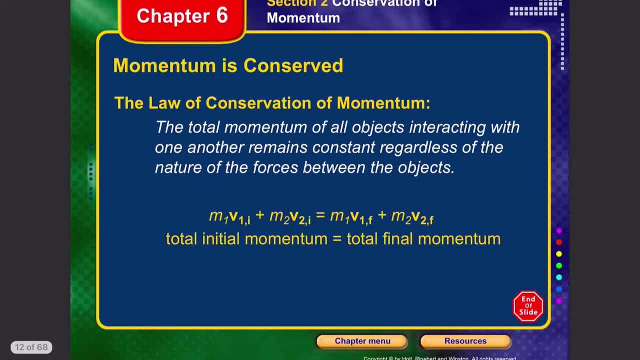 Compare the total momentum of the object to the change in momentum of the object, So the total momentum of two objects, state the law of conservation of momentum And finally predict the final velocities of objects after collision, given the initial velocities, force and time. So let's start with the law of conservation of momentum. So what does the law of conservation 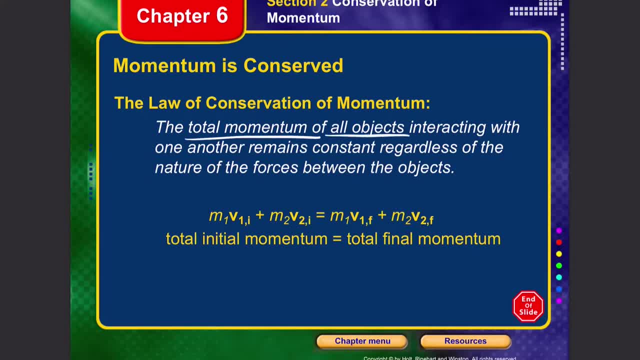 of momentum say So. it says that the total momentum of all objects interacting with one another remains constant, regardless of the nature of forces between those objects, Which means that the total initial momentum is equal to the total final momentum. So when you have two bodies, let's say, for example, you have two objects, You have two objects, You have. 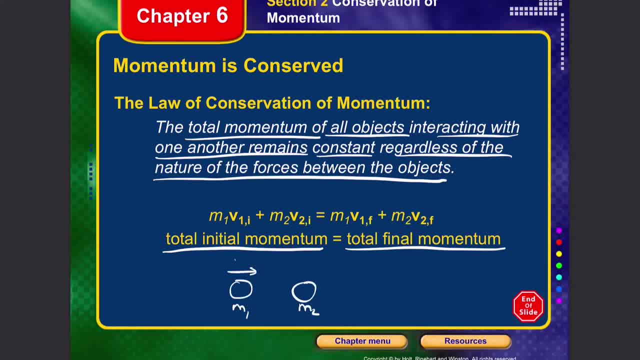 an object. you have an object And then the final velocity will be, say, for example, YM1 and mass YM2.. Let's say, we're traveling with the initial velocity of V1i and this is traveling with the velocity of V2i. Now, provided that they collide, then the so when? 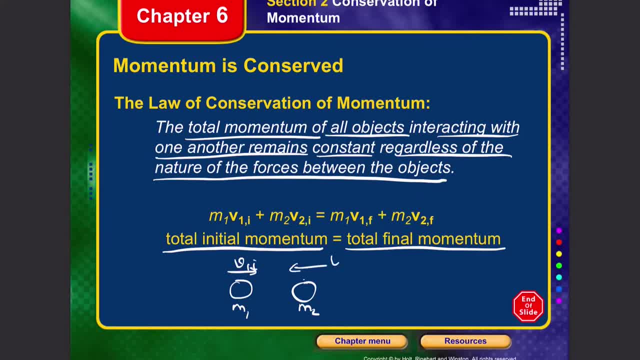 they do collide. let's consider that if they do collide, then their final velocities. so then their final velocities will be: let's say, for example, this is V1f and this value will be V2f, still M1 and M2.. Now the amount of initial momentum is M1, V1i plus M2- V2i. 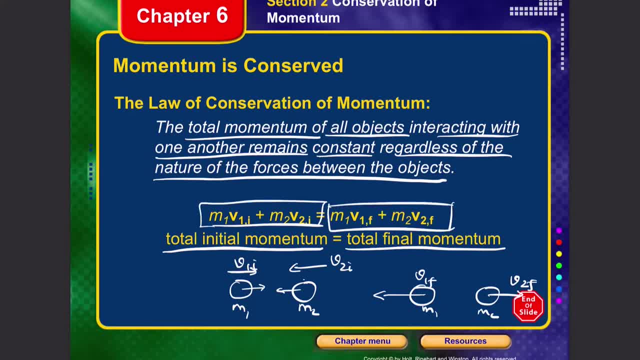 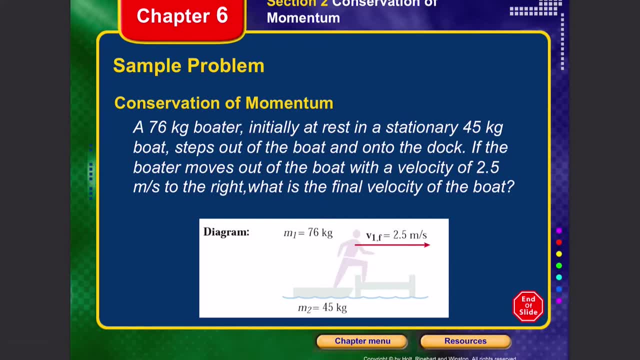 is equal to the total momentum, the final momentum, which is M1 V1f plus M2 V2f. So let's take an example problem and try to solve this and understand how momentum works. So what is given here? a 76 kg boater initially. 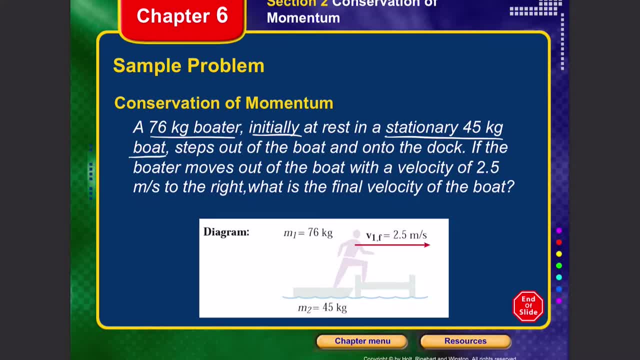 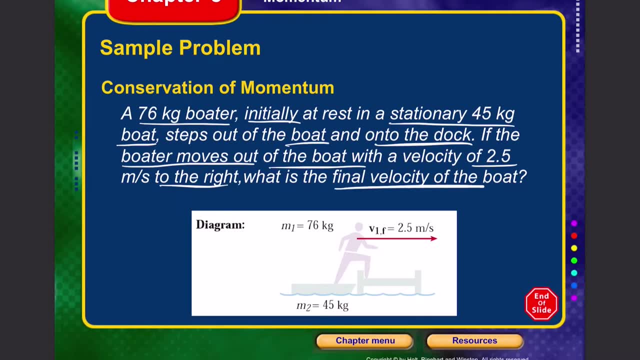 rests in a stationary 45 kilogram boat, steps out of the boat onto the dock. if the boater moves out of the boat with the velocity of 2.5 meter per second to the right, what is the final velocity of the boat? Now notice the diagram here shows. 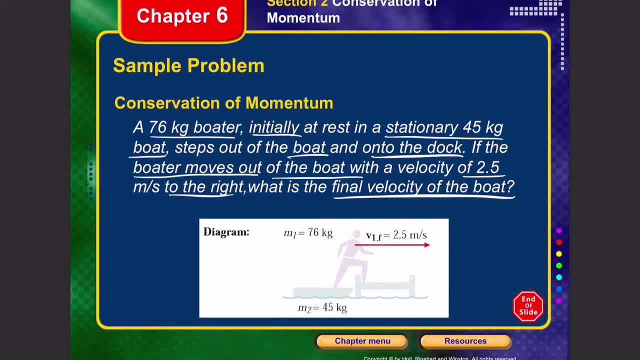 you the actual finish scenario. so this is the person, this is the boat right here and you have the person on the dock. Now, initially, there is no momentum for the boat, no momentum for the person. but when the person starts moving, what will happen is that he tries due to the friction, he pushes this in the opposite. 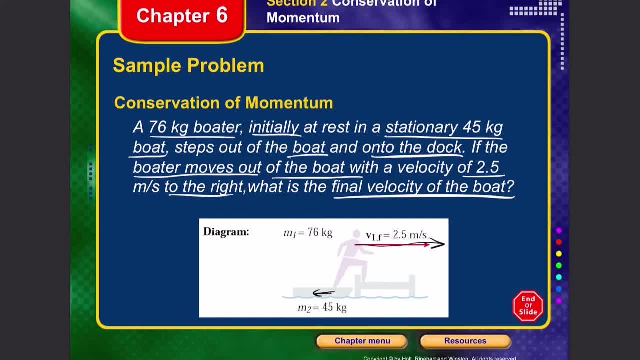 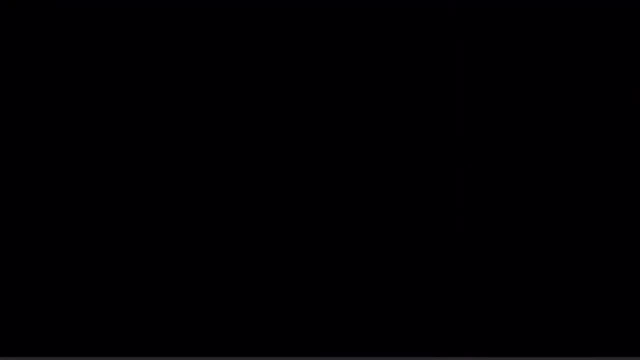 direction, resulting in a momentum in the final velocity. So they are asking you to find V2f. so they are asking you to find V2f now. let's use the momentum situation right now. so what do you have here? you have M1, M2. so let's consider: this is the man. 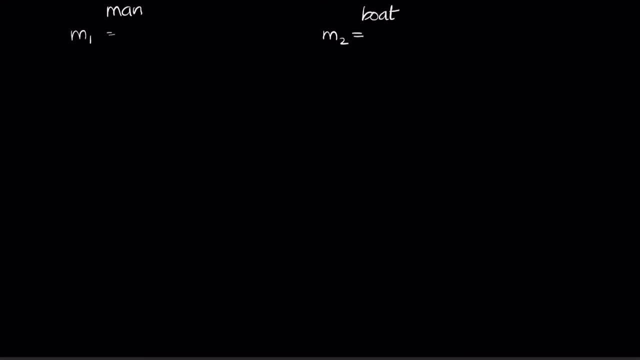 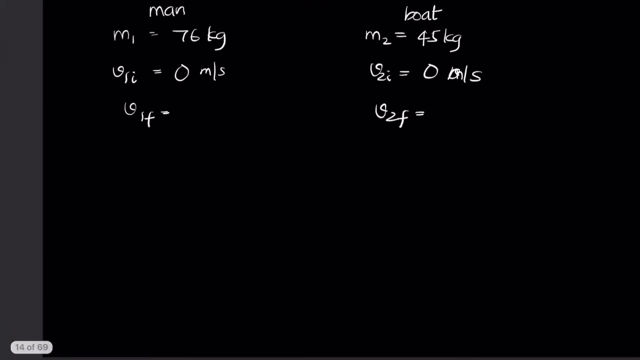 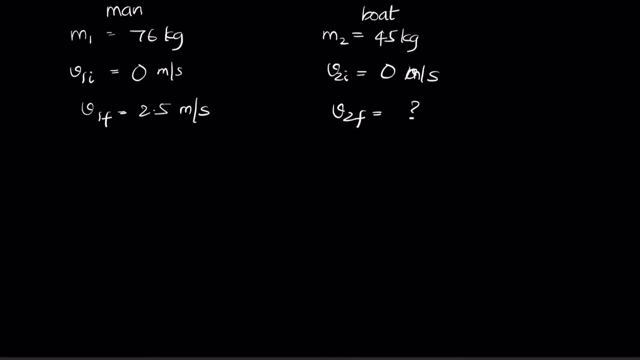 and this is the boat. so the man has a weight of 76 kilograms. the boat is 45 kilograms, which is not kilograms. initially they are not moving, so both of them have zero meter per second velocities, initial velocities. then the man moves with the velocity of 2.5 meter per second and we have to find v2f. so again, the law of 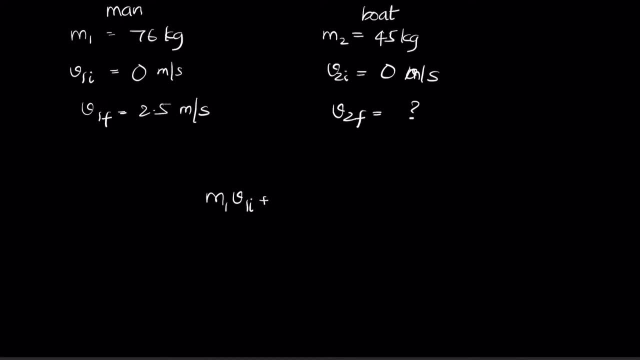 conservation momentum says that the m1 v1i plus m2 v2i equals m1 v1f plus m2 v2f, so which is gonna be? the m1 is 76 times 0 plus 45 times 0 equals 76. 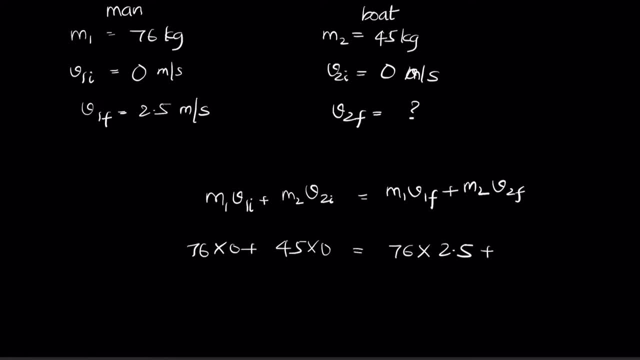 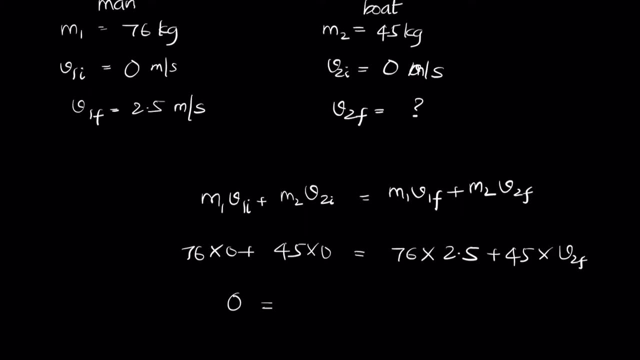 times 2.5 plus 45 times v2f. so this is 0 equals 76 times 2.5 plus 45 times of VF. so now we are going to look at the total velocity of the system and we need to write down: 45 times VF equals minus 76 times 2.5. divided by so VF becomes 76. 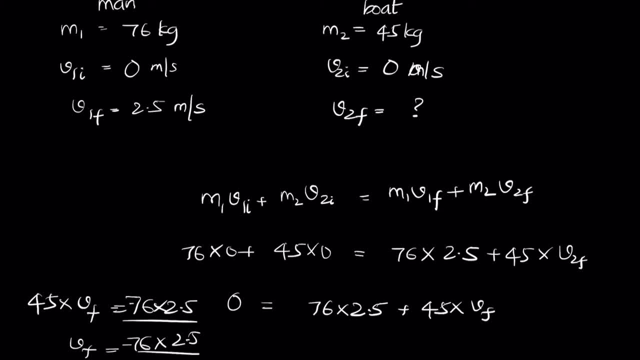 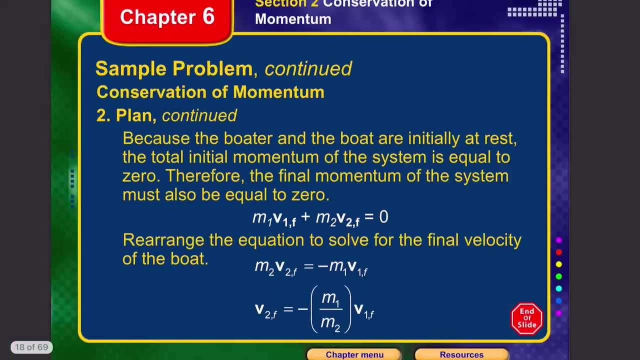 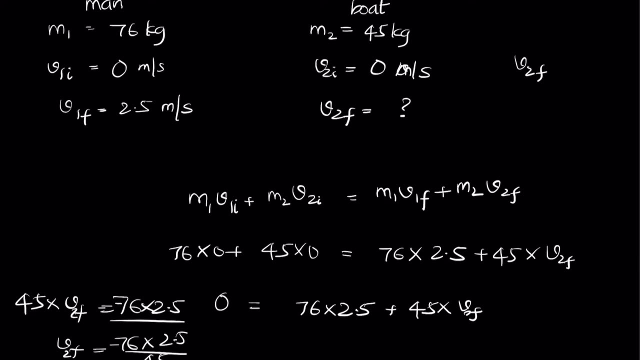 times 2.5 divided by, so minus 76 times 2.5 divided by 45. so when you calculate the final value, that value will become minus 4.2 meter per second. so V to F here is minus 4.2 per second. now the minus here represents that 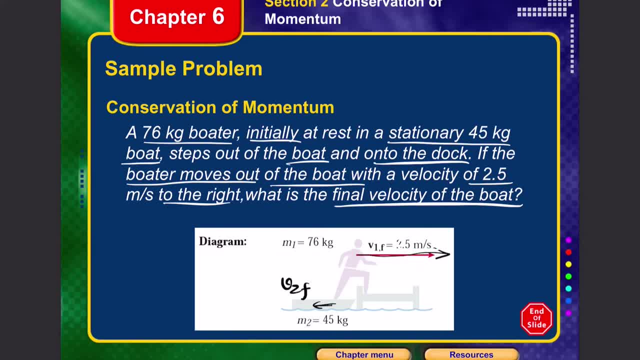 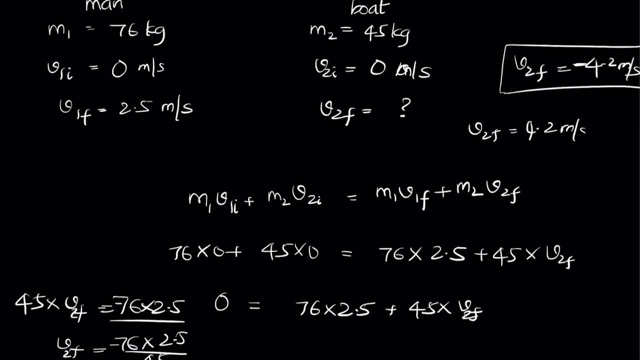 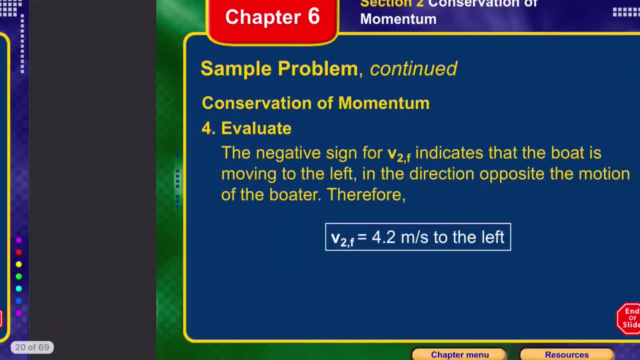 notice that the person is moving to the right. so it means that the work is gonna go to the left. so this is the direction. so, which means V to F is 4.2 meter per second through the left. so that's the negative direction. that's what it means by the negative sign right there now. next, let's take 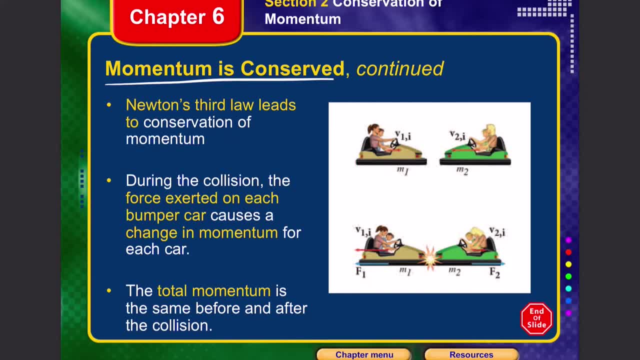 interaction, which is the negative sign right now, and look at the next. let's take interaction, which is the negative sign right now, and look at the next. let's consideration what others can be considered as conservation of momentum. so one of the main ones that can be considered as conservation of momentum: 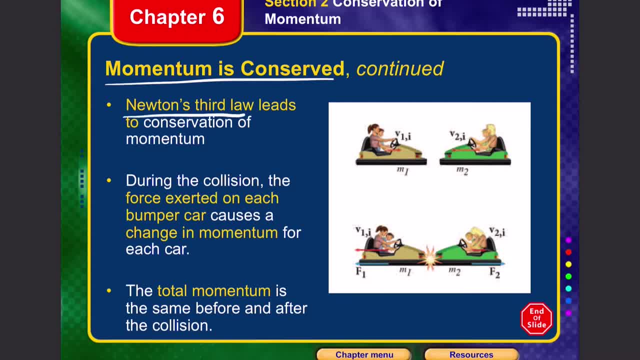 is the Newton's third law. so Newton's third law generally leads to conservation of momentum because the during the collision the force exerted on each of the bumper car here causes a change in momentum of each car, but the total change in momentum is the same before and after collision. because 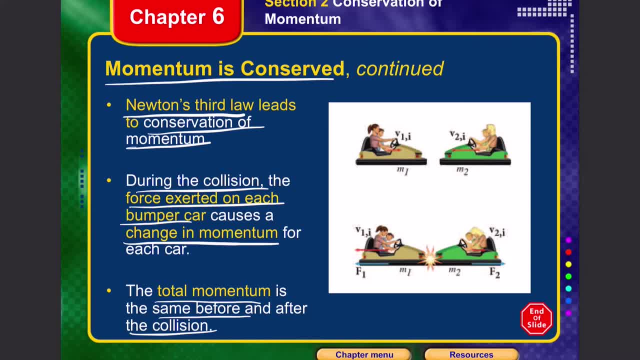 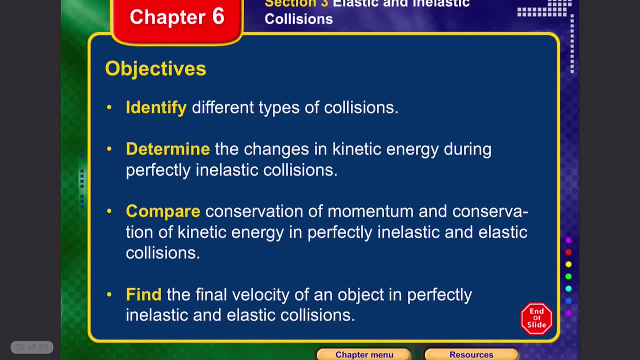 initially the amount of force that so equal cause there is. there is an equal and opposite reaction there, so which means that the force is going to be the same. so with that we end section 2. next let's come to the last one, section 3: elastic and inelastic collisions. so in this section we're going to try to 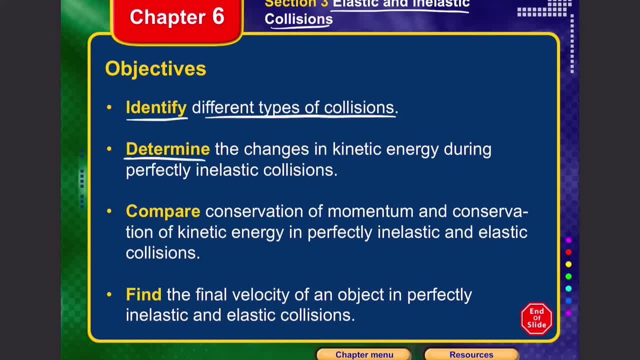 identify different types of collisions. second, we try to determine the changes in kinetic energy during perfectly inelastic collisions. third, try to compare conservation of momentum and conservation of kinetic energy in perfectly inelastic and perfectly elastic collisions. finally, find the final velocity of an object in perfectly inelastic and perfectly elastic collisions. let's start with collisions. so. 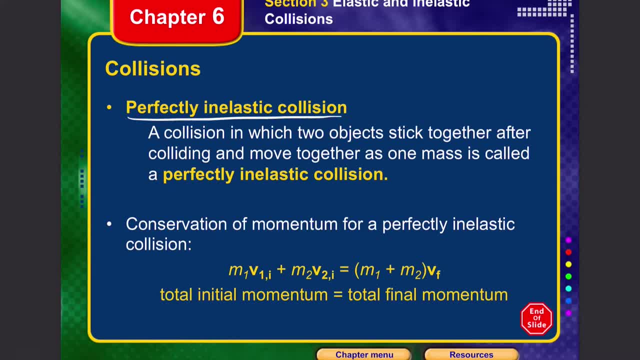 in collisions. let's start with a perfectly inelastic collision. so a perfectly inelastic collision is where a collision, where that the two objects stick together after colliding and move together as one mass, is generally called as a perfectly inelastic collision. an example of this would be a train car, for example, if you see the train engine and a train car. 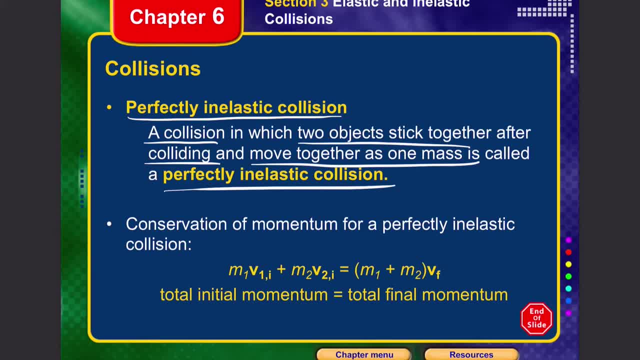 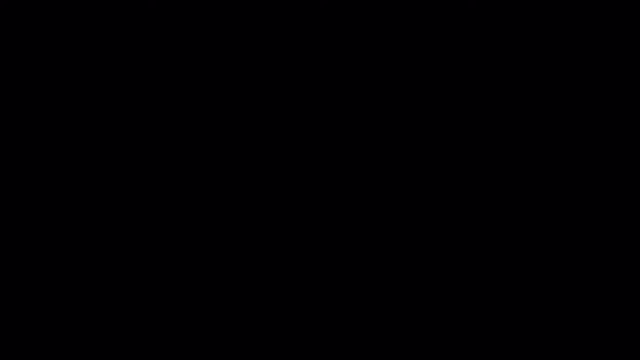 trying to connect each other. once the train engine sticks onto the train I, there becomes one single unit and they travel with a single velocity. so that is the end behind the perfectly inelastic collision. that is an example of a perfectly inelastic in environmental. so what happens there? so let's see, we have a 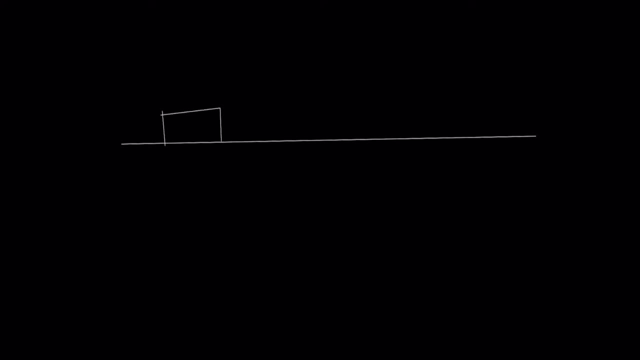 surface. right here and on the surface, we have two bodies: m1 and m.2. let's say this moves with initial velocity of v1i and this moves with the initial velocity of v2i. Now let's see m1 and m2 combine together and undergo a perfectly inelastic collision. So when they undergo perfectly, 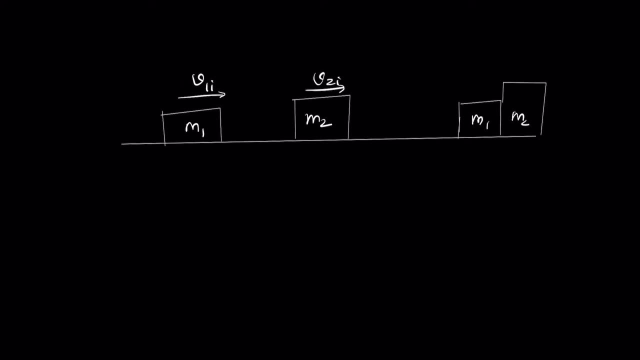 inelastic collision. so what is happening here is that these two are going to stick together and the combined unit now travels at a single velocity of vf. So, based on the situation right here- this is before, and if this is after- we can consider the law of conservation of momentum. 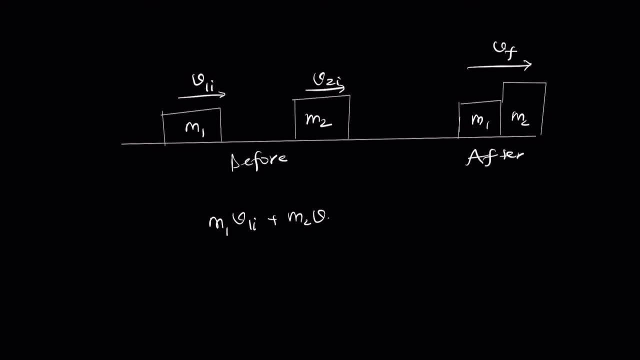 which writes m1 v1i plus m2 v2i equals now the second part. the mass is combined, which means that we can write it as m1 plus m2 times. the velocity is vf. So this here is the equation for a perfectly inelastic collision. So from this we can write the final velocity: vf. 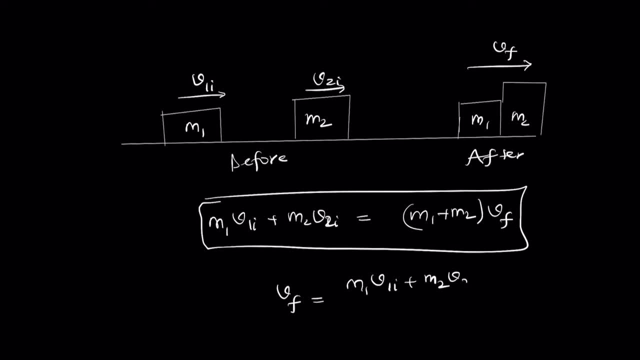 as m1, v1i plus m2, v2i by m1 plus m2. so this is the final velocity, provided we have the initial velocity, and we vanquish this with final velocity, which we can sum up just as v1. so we have the. 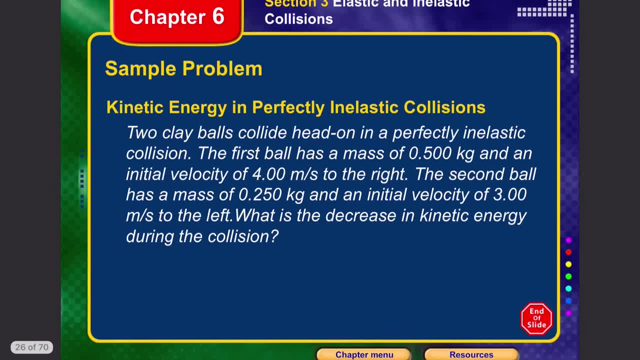 final velocity. you can add the final velocity because if we are saying that, if we are taking velocities of the two objects, So let's take an example problem and try to solve this. So what is given here? You have two clay balls collide head-on perfectly in. 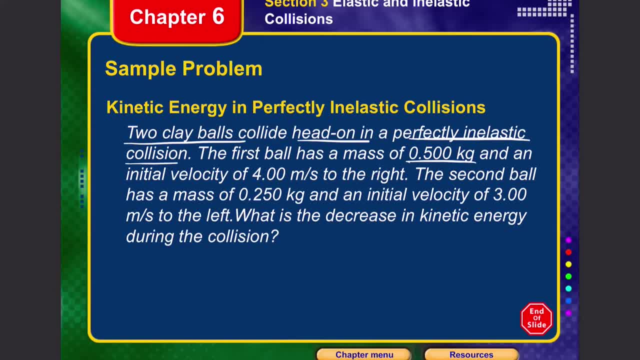 elastic collision. The first ball has a mass of 0.500 kilograms and initial velocity of 4 meter per second to the right. The second ball has a mass of 0.250 kilogram and an initial velocity of 3 meter per second to the. 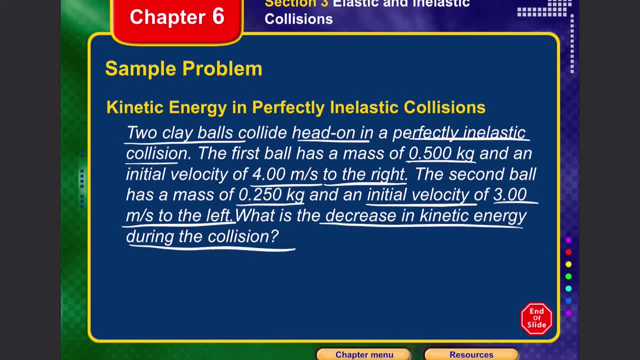 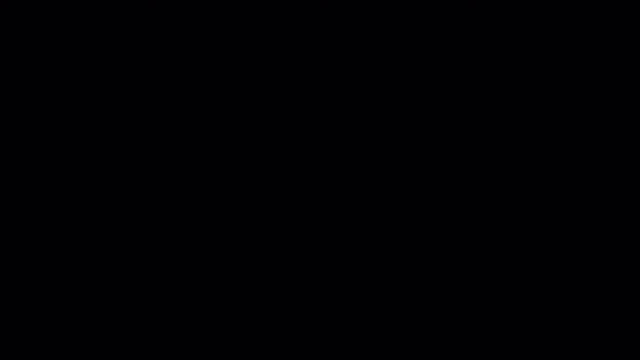 left? What is the decrease in kinetic energy during collision? So first things first, let's try and find the final velocity, because we need the final velocity to calculate the change in kinetic energy. So first write down the data. what is given? So the first ball has a mass of 0.500 kilograms and 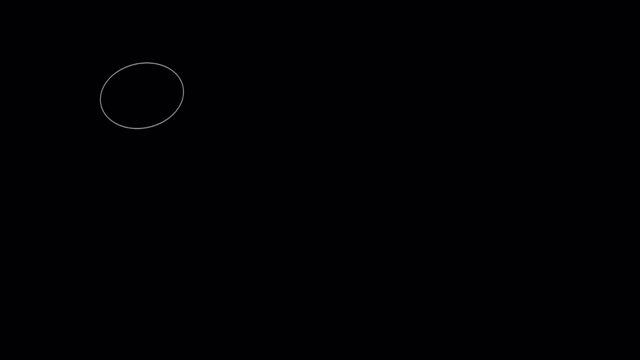 initial velocity to the right. So let's say this is the first ball and this is the second ball right here and this has a mass. this is m1 and this is m2.. So m1 here is 0.500 kilogram and it has a velocity of 4 meter per second to. 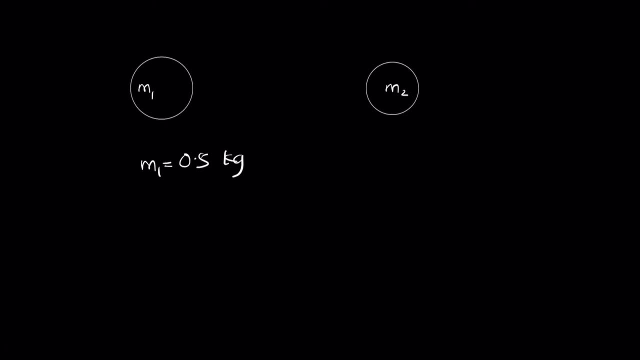 the right. So, for example, this is the body right here. it moves to the right, and m2 here is moving towards the left. So this travels at a velocity of 4 meter per second and m2 here is traveling the opposite direction with a velocity of 3 meter per second. 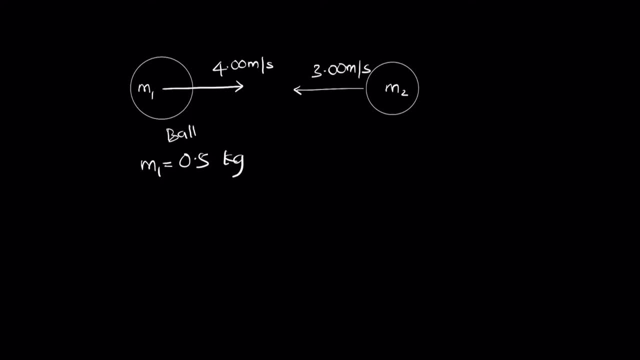 So let's consider this as ball 1 and let's write ball 2.. m2 is 0.250 kilogram. Now v1 can be written as 4 meter per second. remember that this is to the right, so which means this is positive, but v2 is towards the left, so 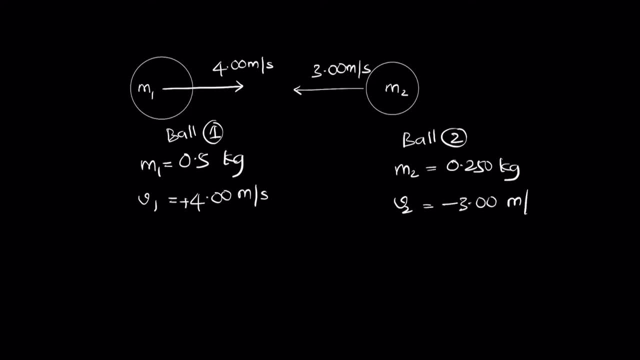 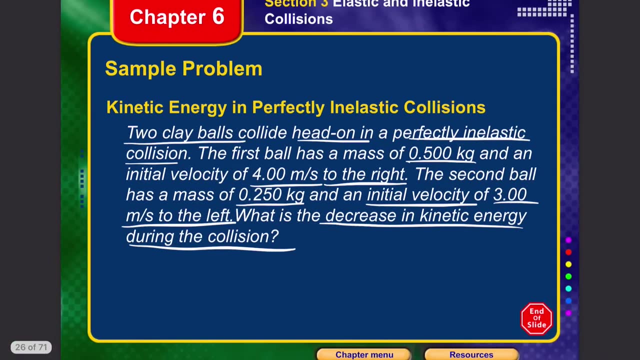 it can be written as negative. so negative 3 to 0.200 meter per second. Remember that whenever you see the signal, whether you see the sign for velocity, you have to mention the direction, because without mentioning the direction we cannot judge the problem. 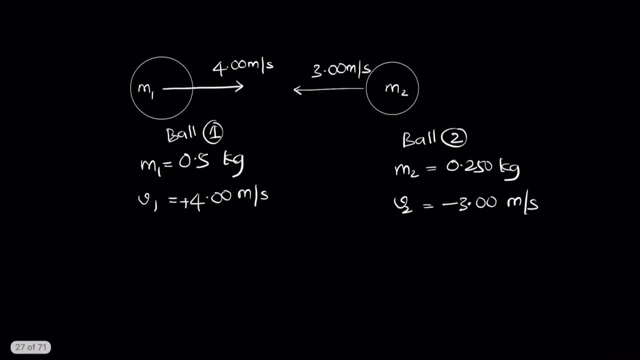 Now they're going to stick together because it's a perfectly inelastic pollution. so from that we can write m1- v1 i plus m2- v2i. this way, this is v1i. v2i is equal to m1 plus m2 times vf. 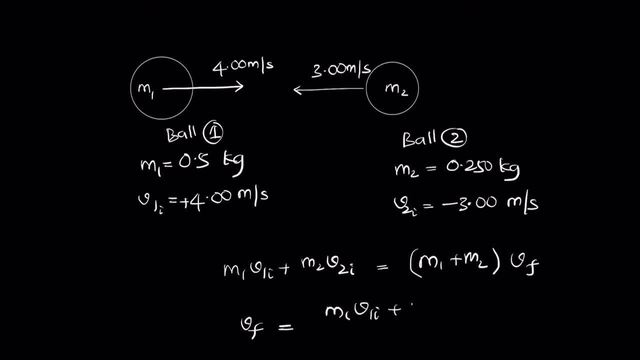 First let's find vf. we have everything that we need. so m1, v1i plus m2, v2i by m1 plus m2. so m1 is 0.5 times v1i, is 4 plus m2, is 0.250 times negative 3 divided by m1. 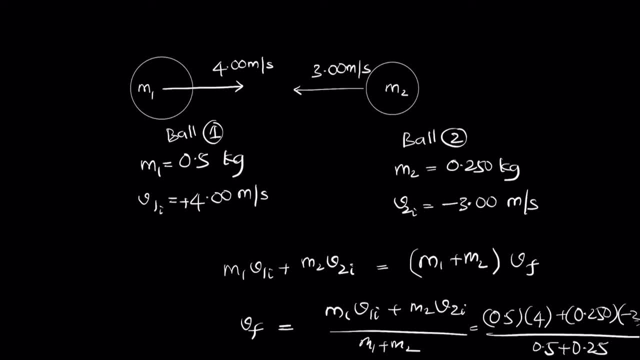 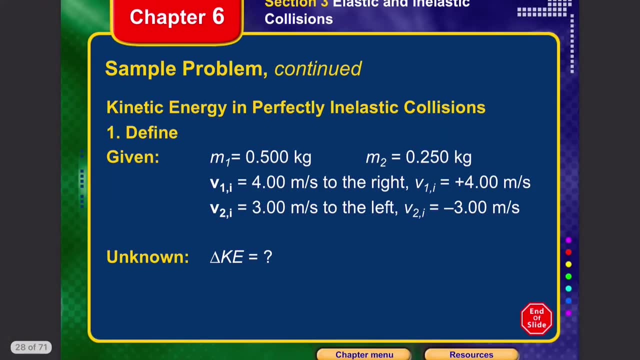 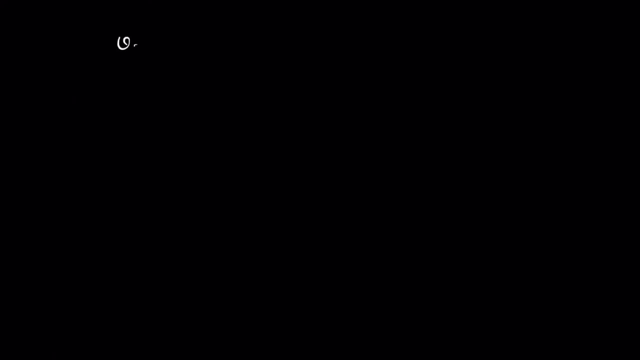 plus m2 is 0.5 plus 0.25.. So from this calculated value we can write that vf is 1.67 bit per second to the right. Now they are asking us to calculate the change in kinetic energy. so which is the final kinetic energy? 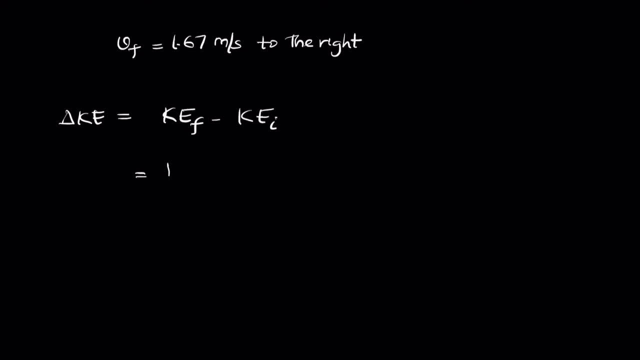 minus the initial kinetic energy. So the final kinetic energy is the total mass, which is m1 plus m2 times velocity square minus initial kinetic energy, is half m1 v1i square plus half m2 v2i square. So half times m1 is 0.5 plus 0.25 times 1.67 square minus of half times 0.5. 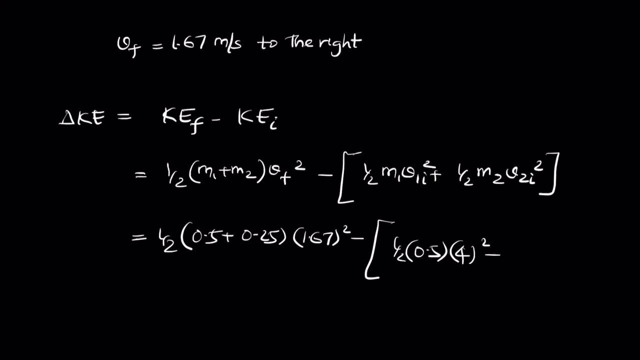 plus 0.25 times 1.67 square, minus of half times 0.5 plus 0.25.. So this is the final kinetic energy times 4 square plus half times 0.25, times negative 3 square. So we can write that this is 1.05 minus. 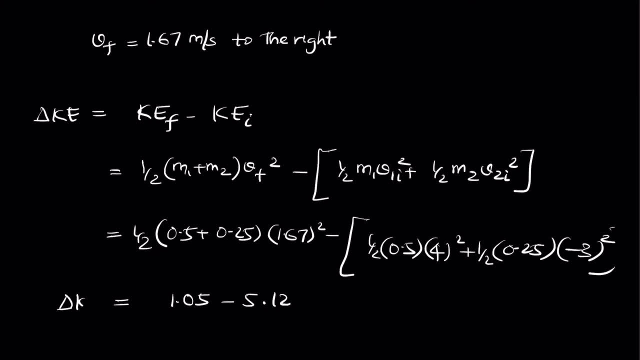 5.12.. So this is delta Ke. So this value becomes minus 4.07 kilojoules or kilojoules joules. So notice that the change in kinetic energy is negative. So which means that here notice that in 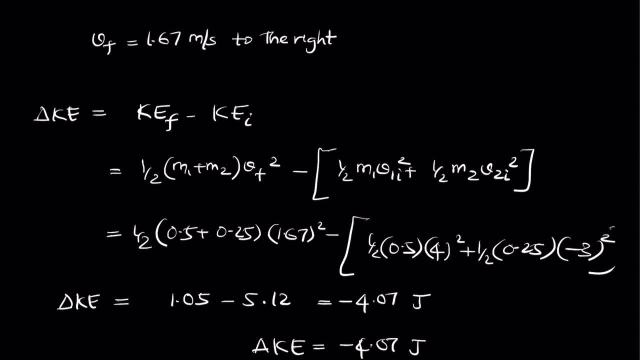 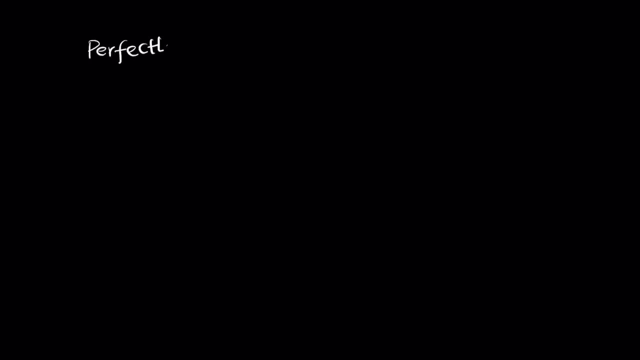 so there is a loss of kinetic energy. from the initial value to a final value There is a loss of kinetic energy. So this brings us to the point about perfectly inelastic collisions. So in a perfectly inelastic collision, momentum is conserved But kinetic energy is not conserved. This is going to be important to 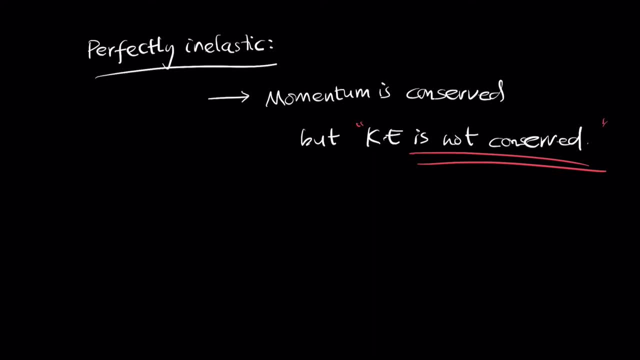 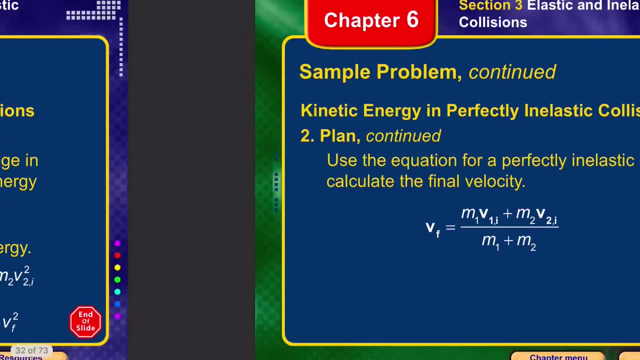 remember that in a perfectly inelastic collision, kinetic energy is not conserved and you will have a loss of kinetic energy in the form of heat or any other force, any other energy. Next, let's talk about elastic collisions. So let's talk about elastic collisions. So let's talk about elastic. 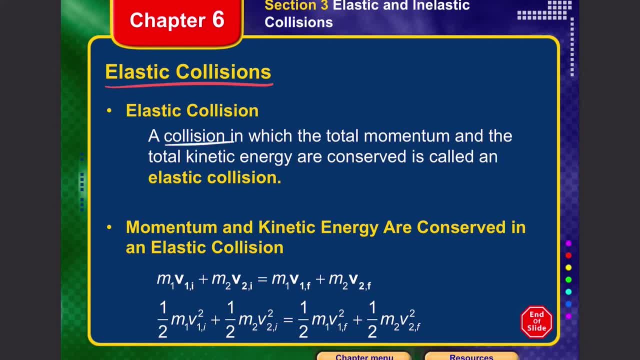 collisions. So elastic collisions is a collision in which total momentum and the total kinetic energy are both conserved. We call that an elastic collision. So what are the two things that are conserved? First, we can write the conservation of momentum equation, And also we can write the 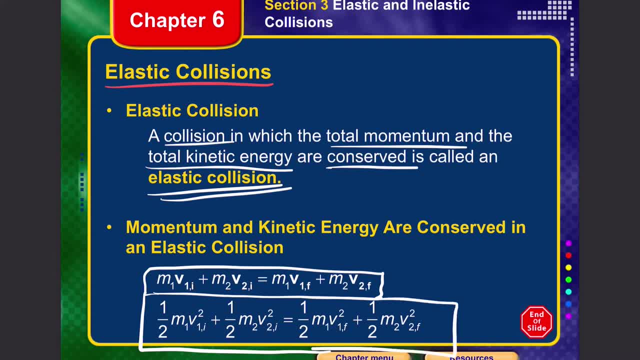 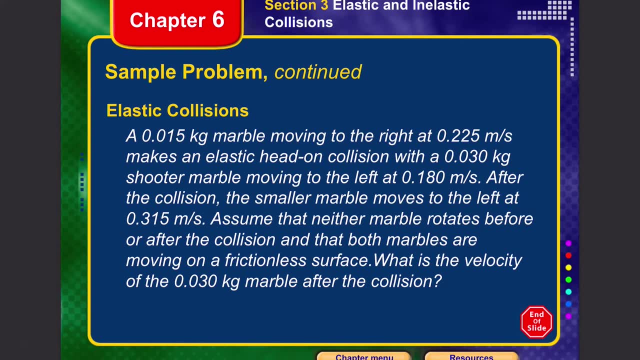 conservation of kinetic energy equation, which is, the total initial kinetic energy is equal to the total final kinetic energy. So Pi equals Pf and Kei equals Kef. The initial kinetic energy is also equal to the final kinetic energy. So let's take an example problem. So what is given here You have. 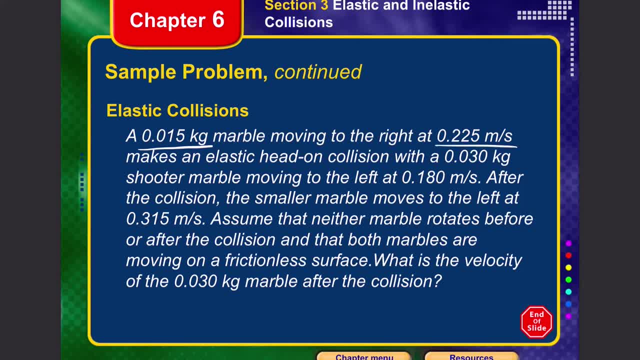 a 0.015 kilogram marble moving to the right at 0.225 meter per second and makes an elastic head-on collision with a 0.030 kilogram shooter marble moving to the left at 0.180 meter per second. After the collision, the smaller marble moves to the left at 0.315 meter per second. 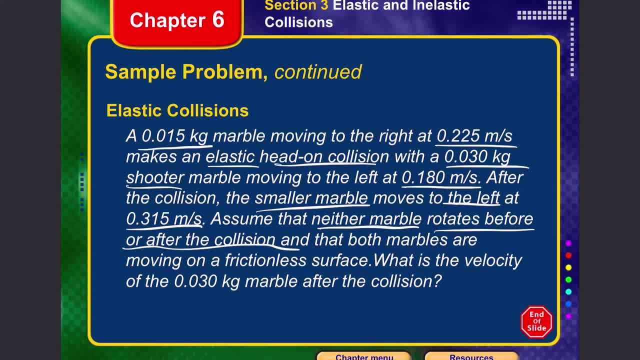 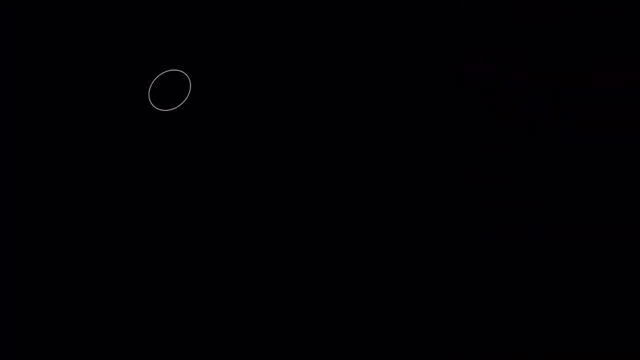 Assume that neither marble rotates before or after collision and that both are moving on a frictionless surface. What is the velocity of the 0.030 kilogram marble after the collision? So now we have two marbles, So let's consider the marble one and marble two. 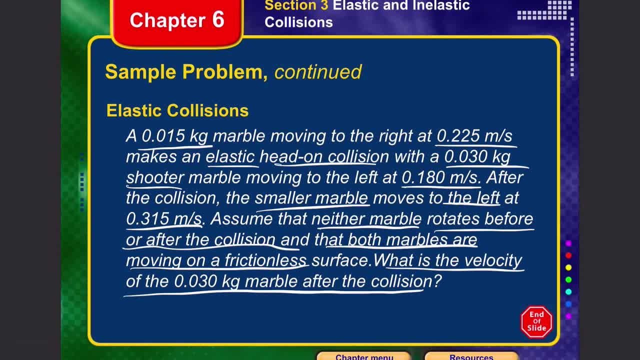 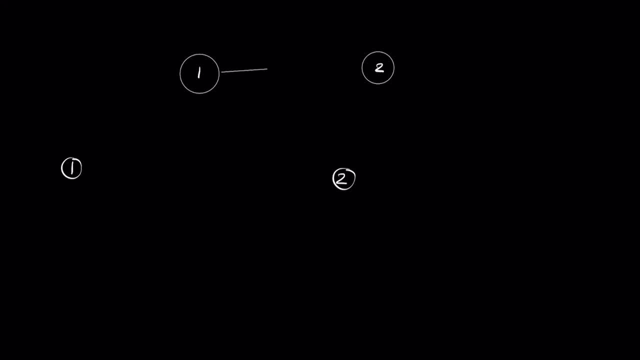 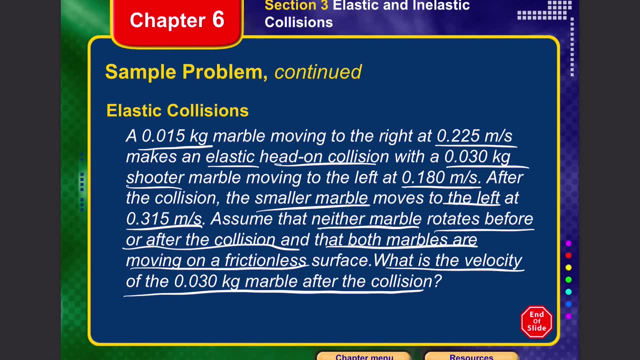 Now the first marble is 0.015 kilogram marble is moving to the right, So this marble right here is moving to the right And this marble is moving to the left, So the second marble is moving to the left. Now the first marble is 0.015 kilogram. 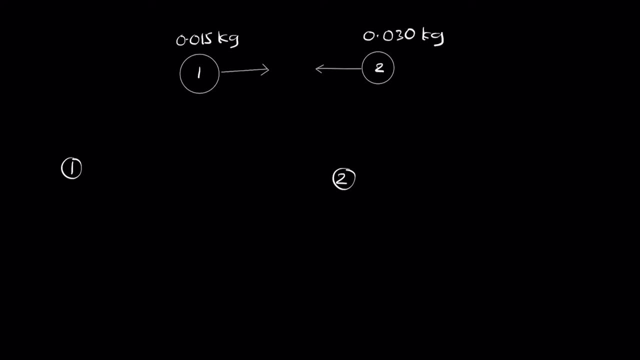 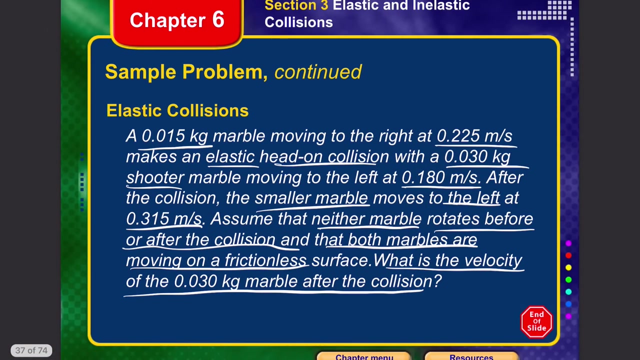 and the second marble is 0.030 kilogram. Let me write this as the bigger marble. So you have two marbles now. Now the 0.015 kilogram marble is moving to the right at 0.225 meter per second. So this moves at 0.225 meter per second, And the second marble is moving at. 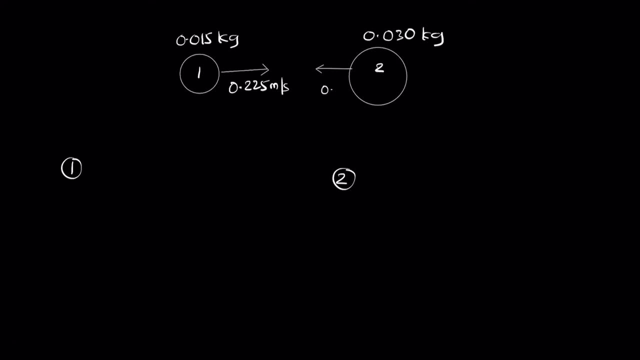 moving to the left at 0.180 meter per second. So this is moving at 0.180 meter per second. So now write down the data: So m1, 0.180 meter per second. So this is moving at 0.180 meter per second. 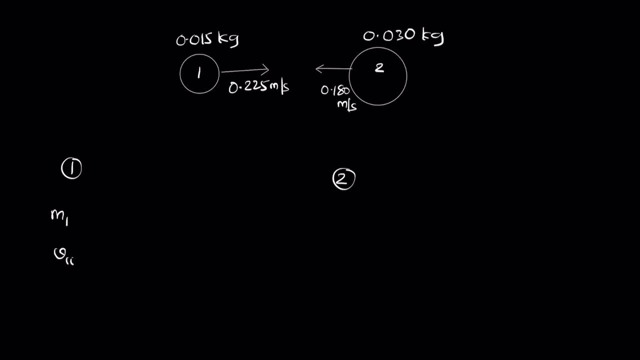 So now write down the data: So m1, 0.180 meter per second. So this is moving at 0.180 meter per second. Now write down the data: So m1,, v1i, v1f, m2,, v2i, v2f. 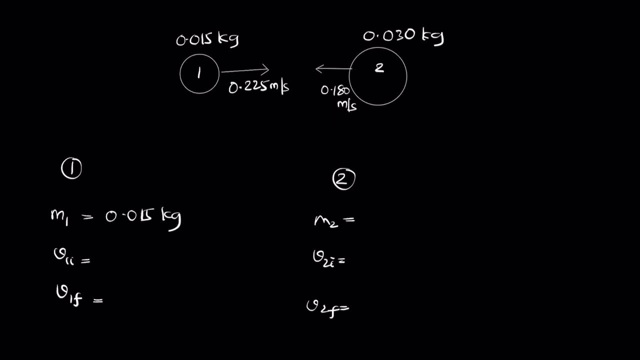 So this is 0.015 kilogram. v1i is 0.225 meter per second. m2 is 0.030 kilogram and this is 0.180 meter per second. Now notice that v2i is in the middle. 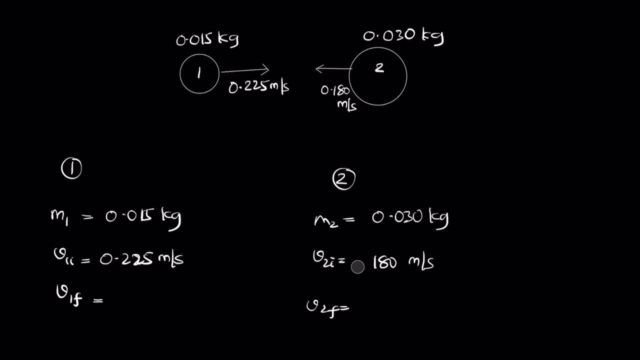 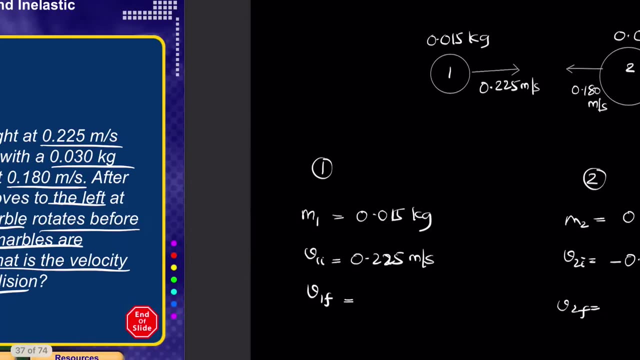 Now notice that v2i is in the opposite direction to that of the v2, v1i, So which means we're going to write it as negative. So, negative 0.180 meter per second. So now what is given at the final part? After the collision, the smaller marble moves to the left. 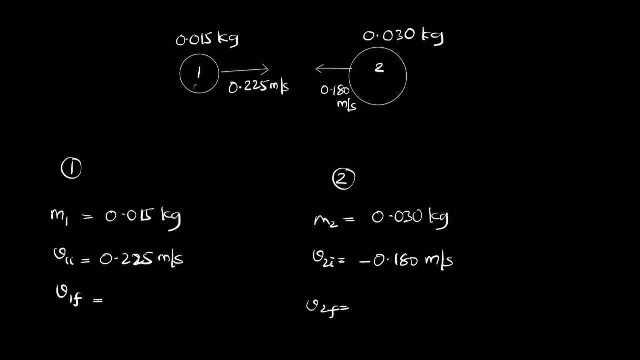 at 0.315 meter per second. So the smaller marble is marble 1.. So it's moving at 0.315 meter per second to the left, So which means that this here is going to the leftward direction, So which can. 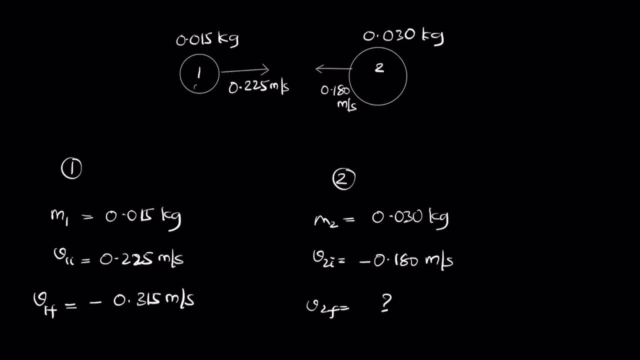 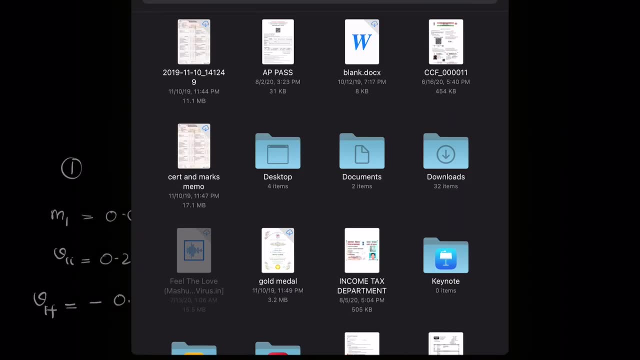 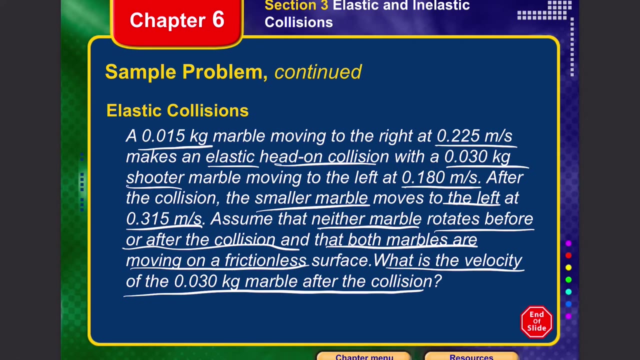 be written as negative. So we want to find v2f Now based on the data. so they are asking us to find. so what is the velocity of the 0.3-3-0 luceu markup? So we are that they're asking us to. 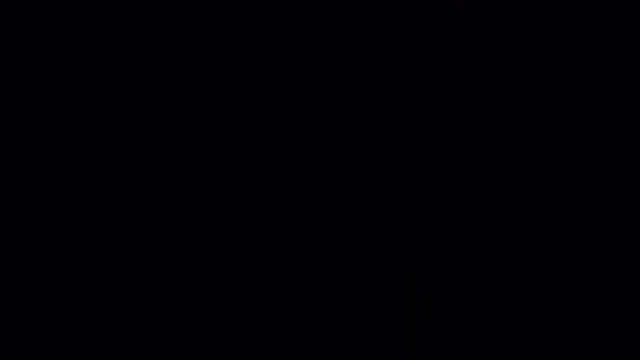 find v2f. So we can use either the conservation of momentum or conservation of kinetic energies. So to make it easier, let's use the conservation of momentum equation. So the conservation of momentum is m1 v1i plus m2 v2i equals m1 v1f plus m2 v2f, so 0.015 times v1i is 0.225. 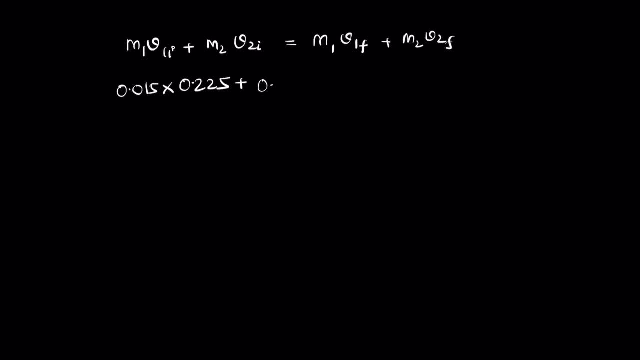 plus m2 is 0.030 times negative. 0.225. 0.180 is equal to m1. v1f is 0.015 times negative. 0.315 plus m2 is 0.030 times v2f plus 0.015. divided by 0.030 equals v2f. so when you reshuffle, this is what you get for v2f now. 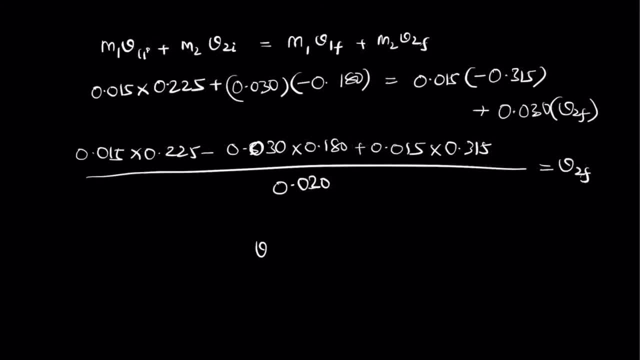 pause the video right here and try to calculate v2f. so when you find the total value, that value becomes 0.09 meter per second to the right. so notice that this is a positive value, so which means that here this is going to be to the right side.